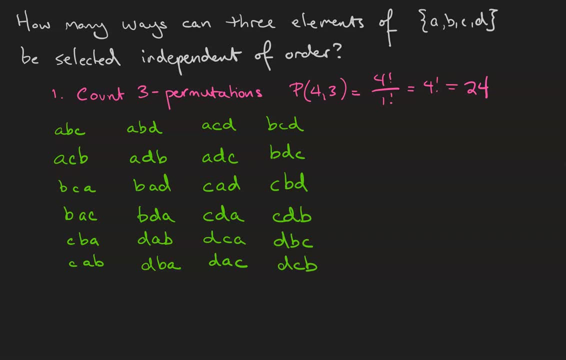 C and D C B. And what we'll notice next is that for each of these three permutations, there are six ways to order it. Notice, for example, that A, B, C, A, C, B, B, C, A, B, A, C, C B A and C A B. 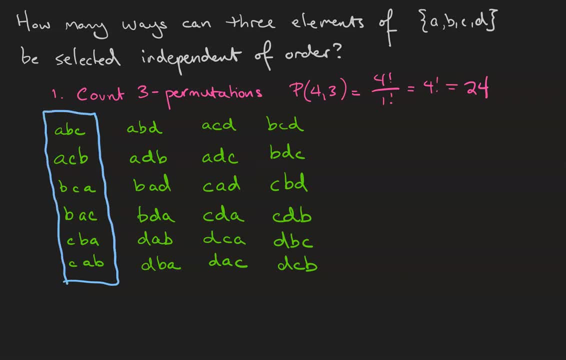 are all the same unordered sample. Likewise with all the permutations of A, B, D, all the permutations of A, C, D and all the permutations of B, C, D. So the next step is to divide by the three factorial orderings for each permutation. So 24 divided by three factorial. 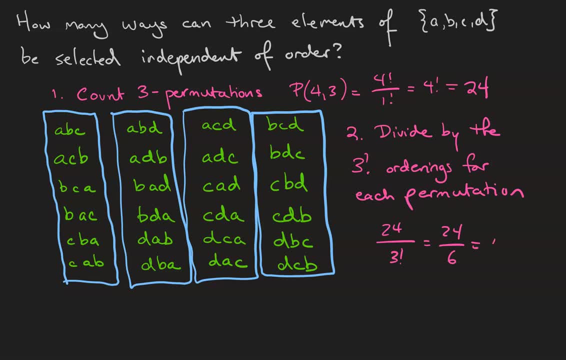 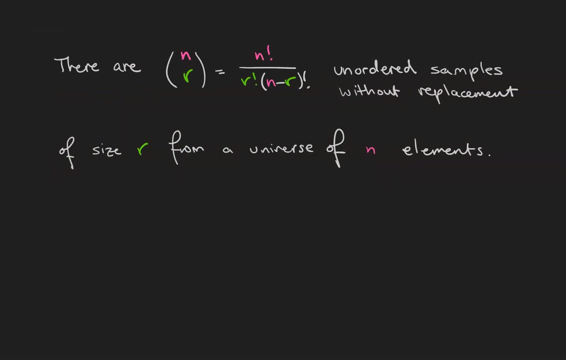 Three factorial is six. 24 divided by six is four And we can count one, two, three, four unordered samples without replacement. So in general there are n factorial divided by r. factorial divided by n minus r. factorial ways to choose an unordered sample without replacement of size r. 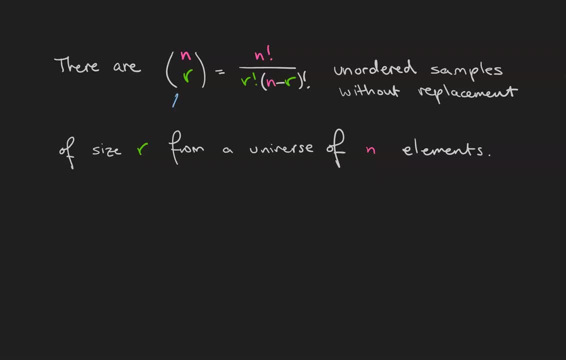 from a universe of n elements. This number is read n, choose r and is called a binomial, A binomial coefficient, for reasons we'll see in the next couple of videos. A key observation is that an unordered sample without replacement is a subset. Notice that the six orderings shown here A, B, C, A C, B, B C A C. B A, B A C. 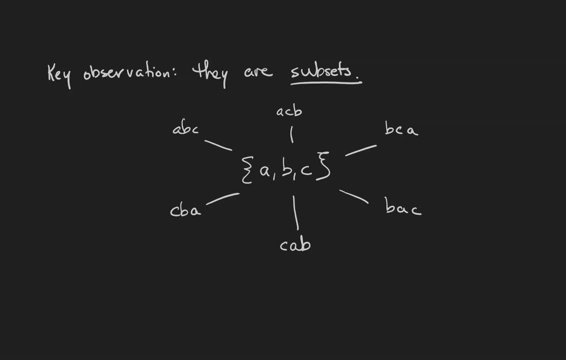 and C, A, B all correspond to the subset A, B, C. once we take away their order To drive this last point home, let's count the subsets of the set A, B, C, D that have sizes Z, Z and Z. 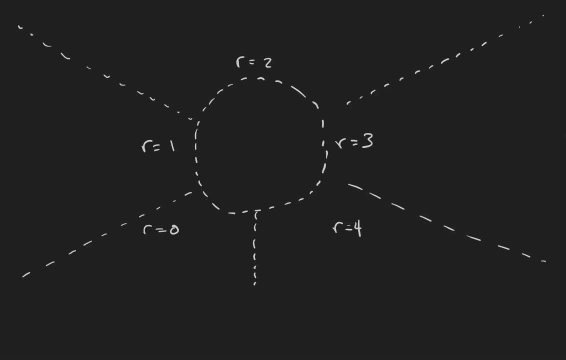 0,, 1,, 2,, 3, and 4 respectively. So when we count the set with size 0, that's just going to be the empty set, And we know that there are only one of those. Well, 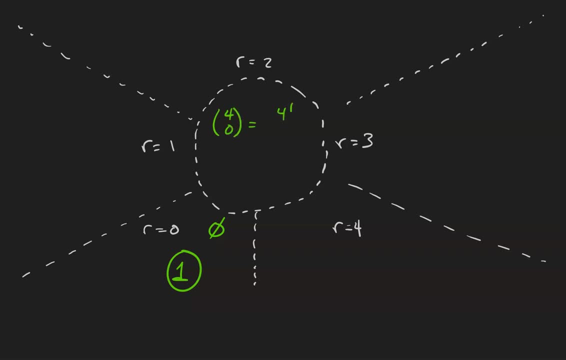 4, choose 0 is the number 4 factorial divided by 0 factorial, 4 factorial. The 4 factorials cancel out and the 0 factorial is just 1, so that counts to 1 as well. Next, when we count the sets that only have one element, we're going to have the set containing A. 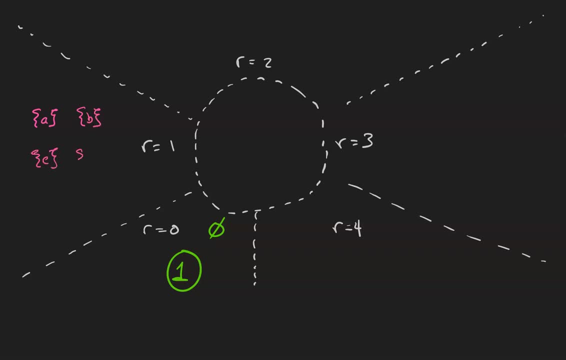 the set containing B, the set containing C and the set containing D, And there are 4. choose 1 of those which is equal to 4 factorial over 1 factorial: 3 factorial. 4 factorial can be written 4 times 3 times 2 times 1 over 3 times 2 times 1. leaves us with just 4.. 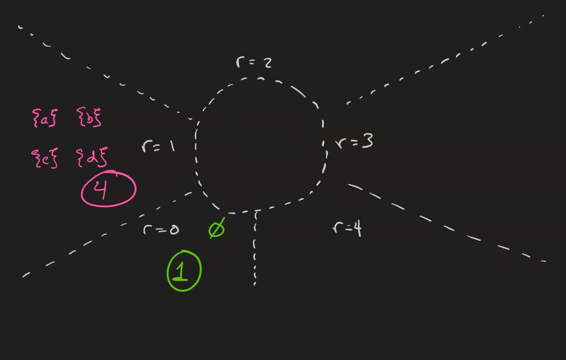 Next let's count these subsets that only have two elements. There's AB, AC, AD, BC, BD and CD. There are 4 choose 2, which is 4 factorial over 2 factorial three times 3 times 4.. So that's 4.. 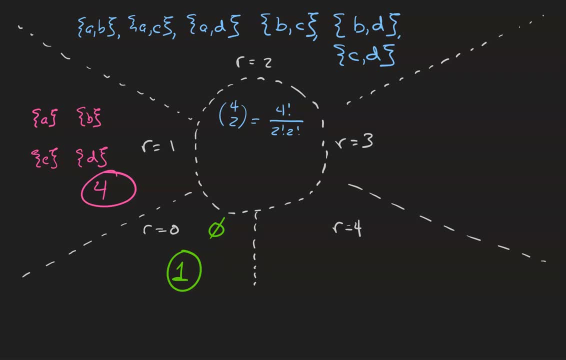 factorial 2 factorial of those 4 factorial is 24, 2 times 2 is 4, and that leaves us with 6, which we've already counted this before, So there's 6 of those. Next let's count the sets that have 3 elements. That's going to be the. 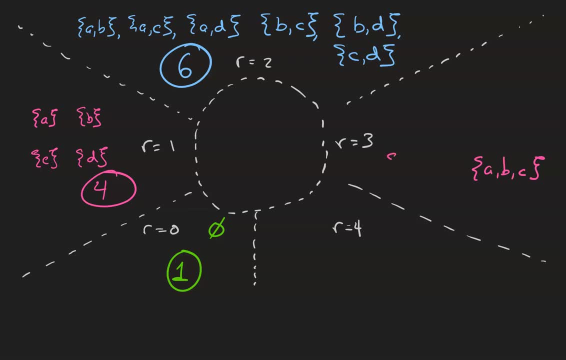 sets A B C, the sets A B D, the sets A C D and the set B C D, And likewise there are going to be 4 of those, because 4 choose 3 is equal to 4 factorial over. 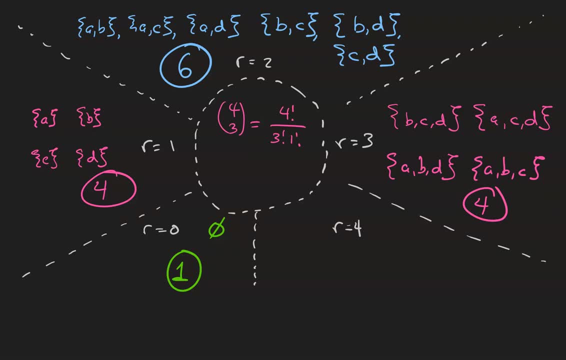 3 factorial- 1 factorial. Now you may have noticed that this is the same as 4- choose 1, because the only difference between the two sets is that the set A only difference is that the order of multiplication in the denominator is different. But there's another reason why these numbers are exactly the same When 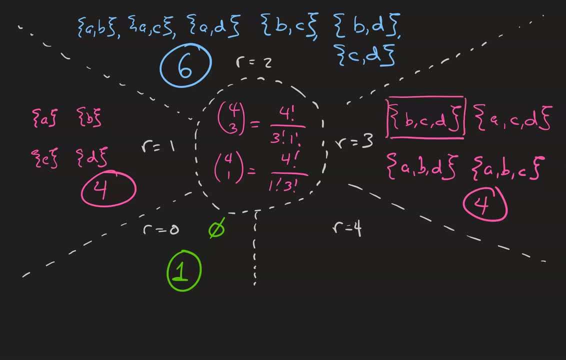 you choose a set with 3 elements from A, B, C, D, you are also implicitly choosing a set with 1 element that you're not going to select. So every 3 element subset of A, B, C, D corresponds to a 1 element subset, and that's why those